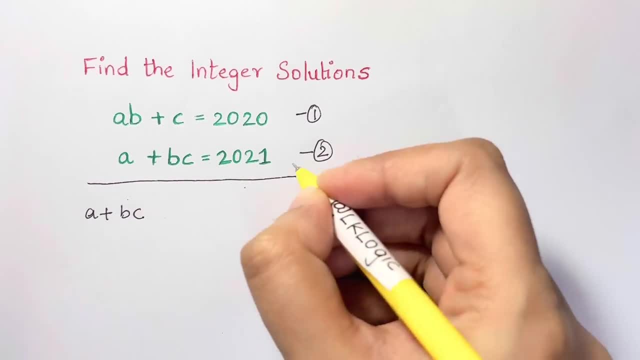 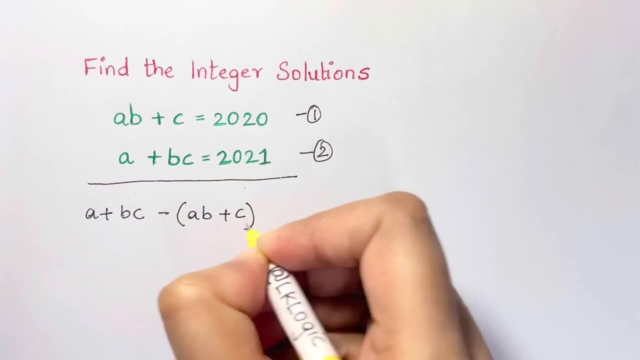 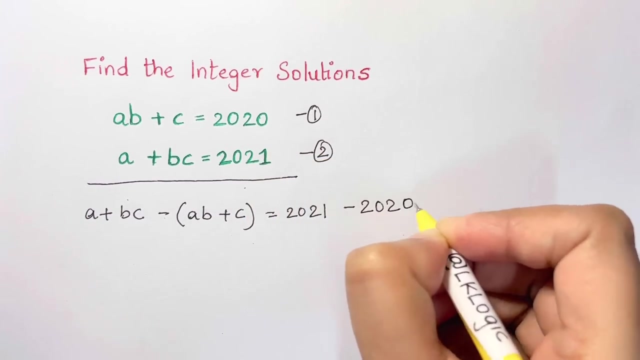 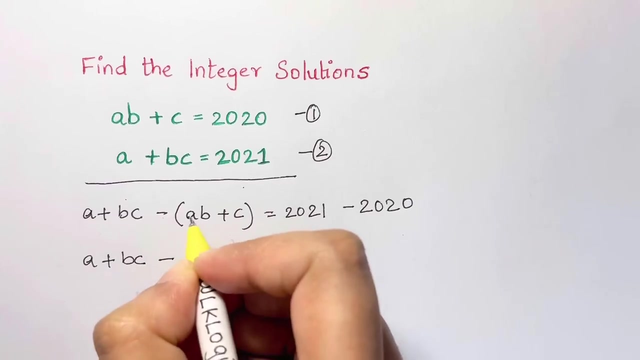 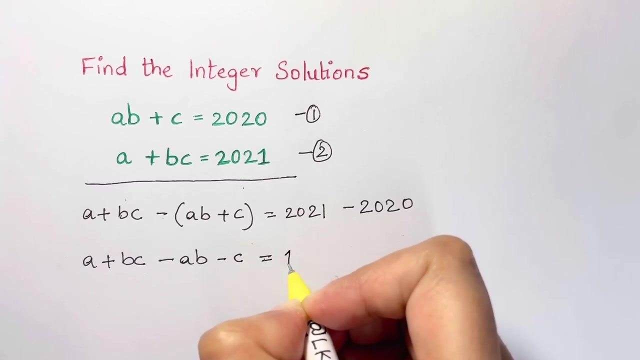 So a plus b c, and then we are subtracting equation one from that, So minus. we have a b plus c is equal to. we'll write down 2021 minus 2020.. That will give us a plus b c minus into plus minus. a b minus into plus minus c is equal to one. The difference 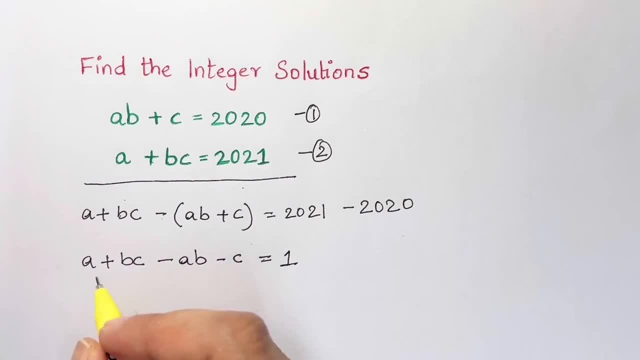 between them is one. Now we have. now let's combine the terms. I can see a and e in this term, So let me write it down together: a minus a, b. then I have plus b, c minus c is equal to one. 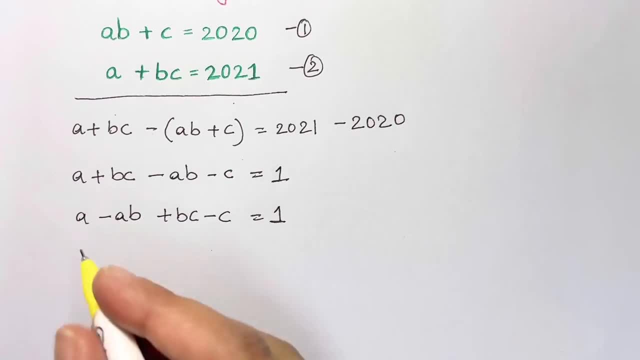 Now what do I do? Here I have a common, The term a here, a here. So let me take it out: common a times one minus b. plus here I can take out c common, So I have: b minus one is equal to one. 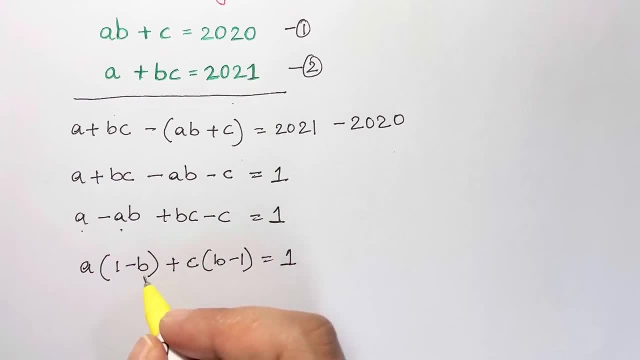 Now what do I see? Here I have one minus b and here I have b minus one. They're not same, There's a difference of signs here. So let me make it similar to that. So I have a into one minus b. 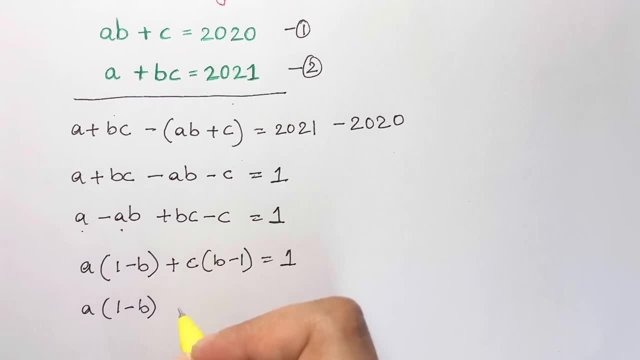 What I'm going to do is take minus one outside. So I have minus one which I've taken outside. Then I have c. Now if I have minus, minus and minus can make this b positive, I'll have to put minus b. 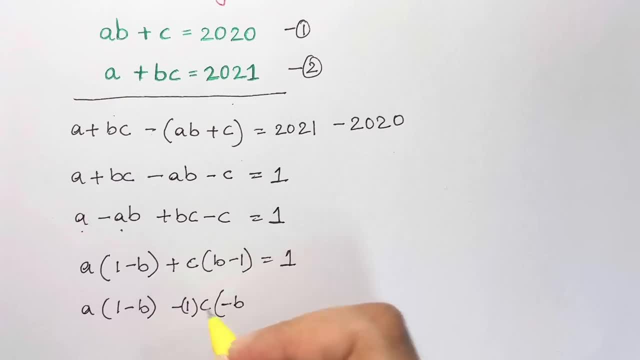 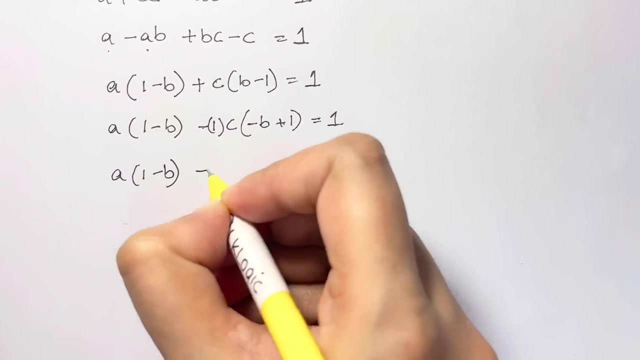 Minus into minus plus b. Now get minus one into something. Something should give me minus one, So that will be plus one. Minus into plus will make it negative. It's equal to one. Now I can write it as: a into one, minus b minus c into one, minus b is. 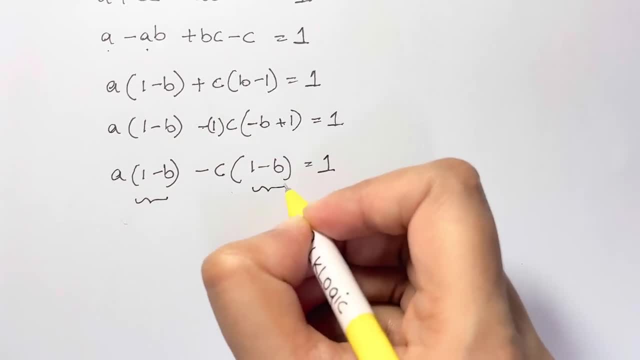 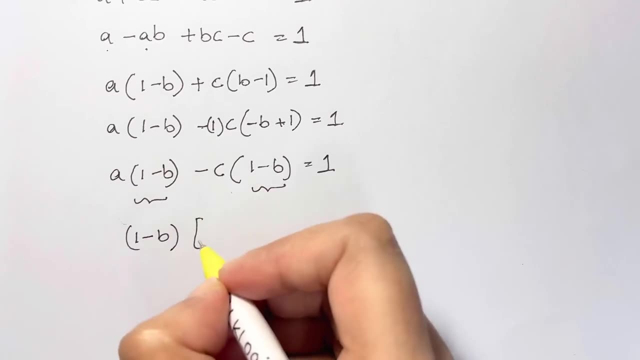 equal to one. Now they are same. These terms are same, So I can take it out as common. So I have one minus b, taken out. Now what is left? a and here minus c, which is equal to one. So I have two factors, One minus b and a minus c. Now we need to find the 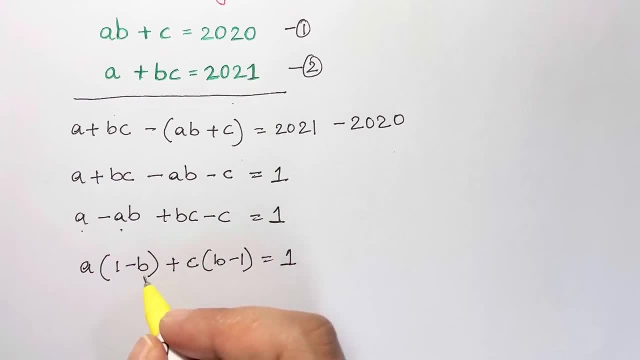 Now what do I see? Here I have one minus b and here I have b minus one. They're not same, There's a difference of signs here. So let me make it similar to that. So I have a into one minus b. 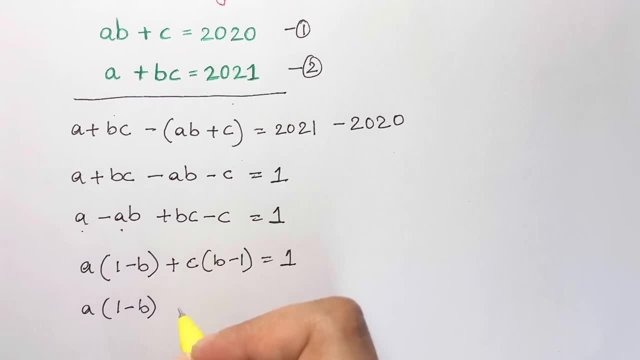 What I'm going to do is take minus one outside. So I have minus one which I've taken outside. Then I have c. Now if I have minus, minus and minus can make this b positive, I'll have to put minus b. 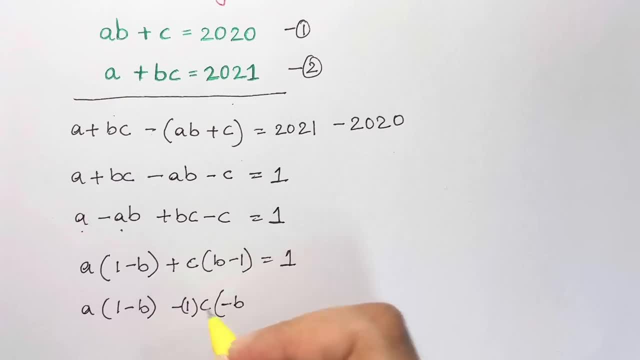 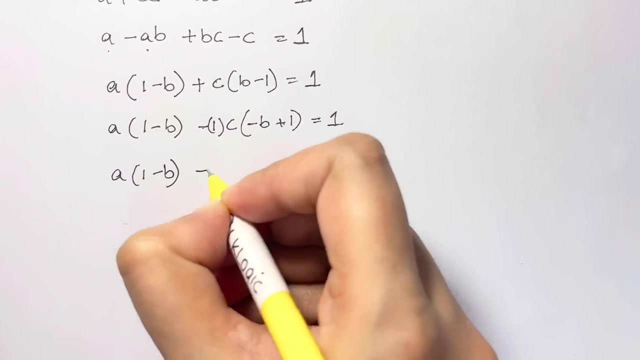 Minus into minus plus b. Now get minus one into something. Something should give me minus one, So that will be plus one. Minus into plus will make it negative. It's equal to one. Now I can write it as: a into one, minus b minus c into one, minus b is. 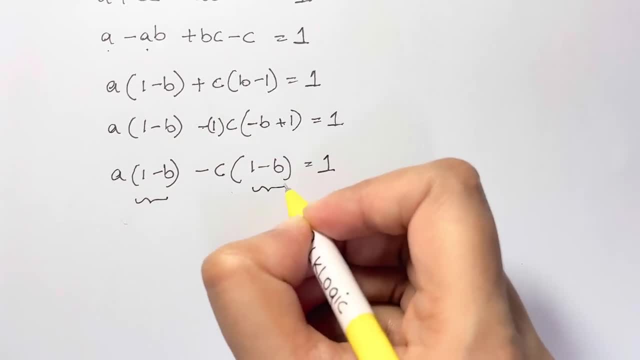 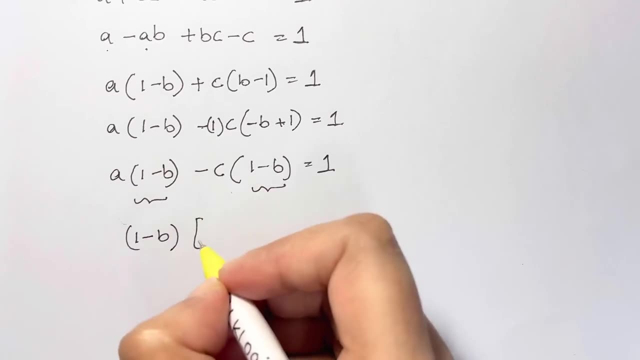 equal to one. Now they are same. These terms are same, So I can take it out as common. So I have one minus b, taken out. Now what is left? a and here minus c, which is equal to one. So I have two factors, One minus b and a minus c. Now we need to find the 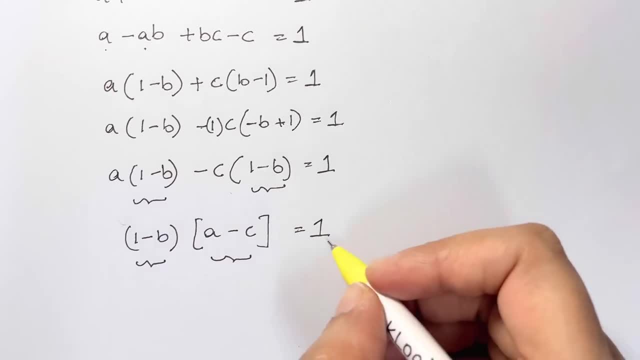 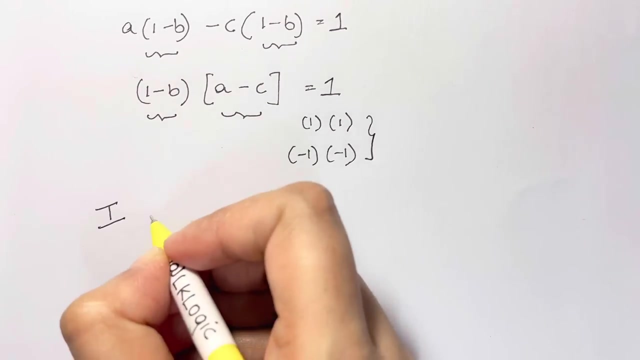 values of a, b and c. So how many solutions can we have Here? there's one, So one is a product of one times one, and it can also be negative one times negative one. So you have two solutions For this. Let's write down the first cases. It will be: one minus b is equal to one and a minus c. 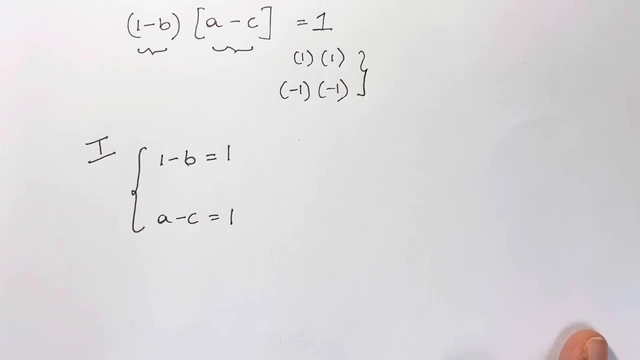 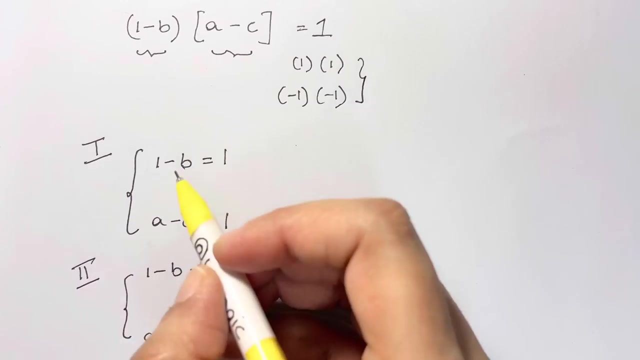 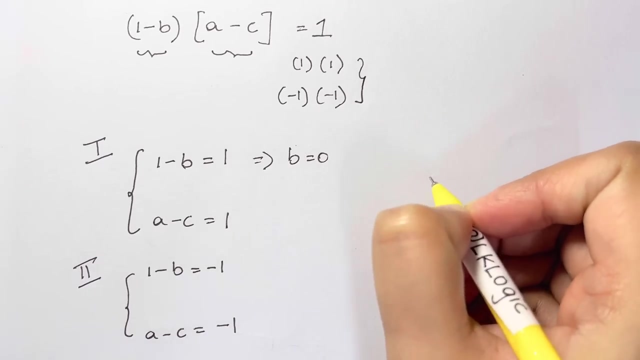 is equal to one. That's the first case, And the second case would be, and the second solution will be, that will be: one minus b is equal to negative one, and a minus c is equal to negative one. One minus b is equal to one. So what do we have? b is equal to zero, And what will be the values of a and c? 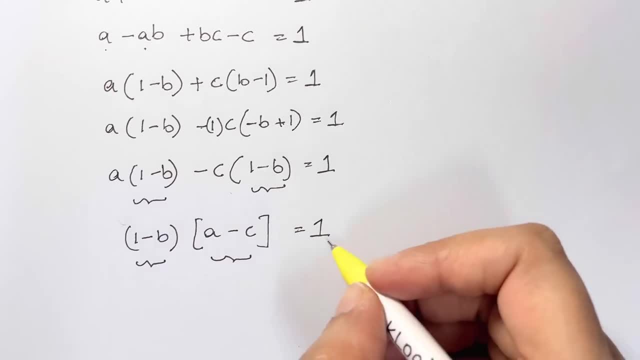 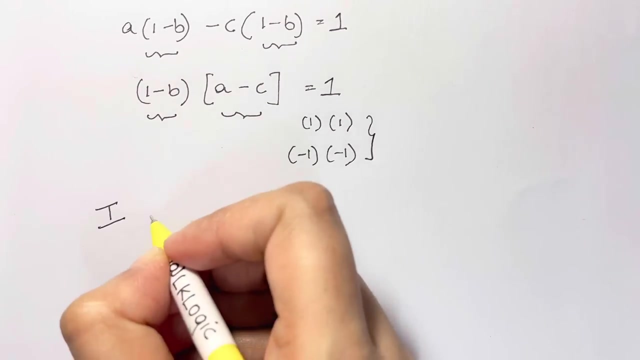 values of a, b and c. So how many solutions can we have Here? there's one, So one is a product of one times one, and it can also be negative one times negative one. So you have two solutions For this. Let's write down: The first case is It will be one minus b is equal to one and a minus c. 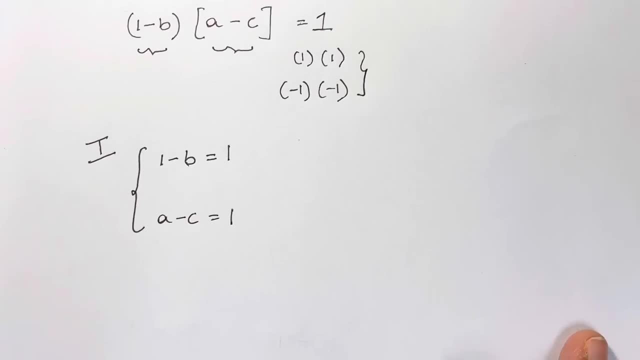 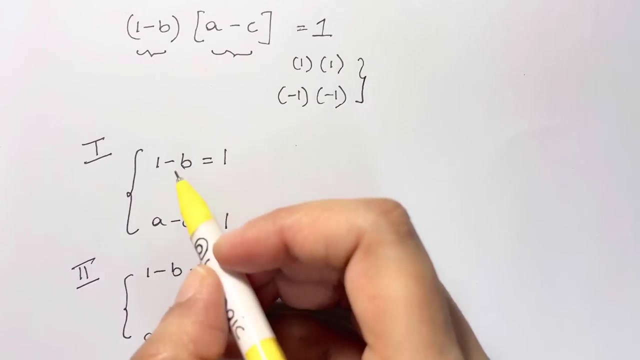 is equal to one. That's the first case, And the second case would be, And the second solution will be, That will be: one minus b is equal to negative one, And a minus b is equal to negative one And a minus c is equal to negative one. One minus b is equal to one. So what do we have? 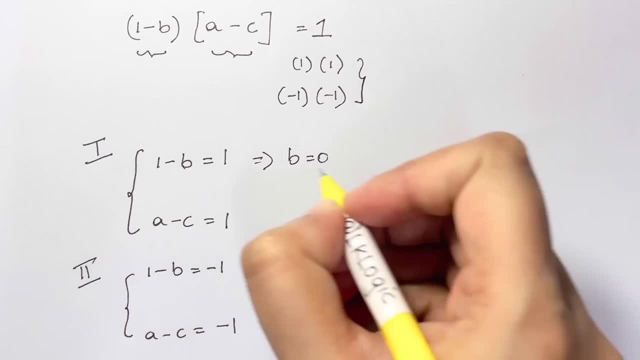 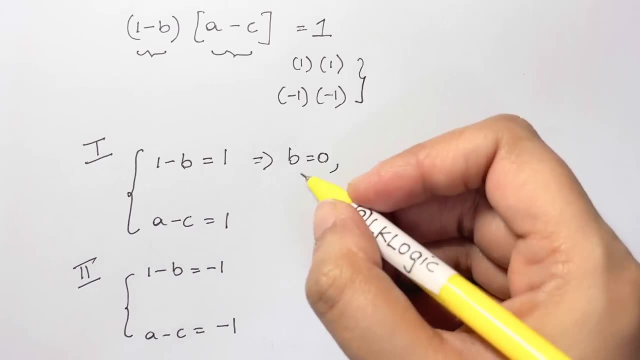 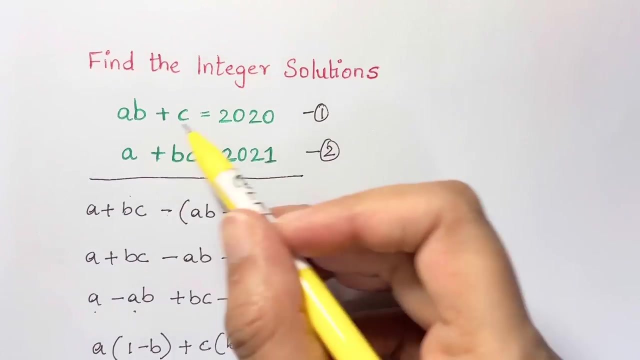 b is equal to zero, And what will be the values of a and c? So for that we need to substitute back the value of b in the equations, Substitute back the values of b in this equation. So let's write it down: a, b plus c is equal to twenty-one. So we have one minus b and a minus c is equal to one. 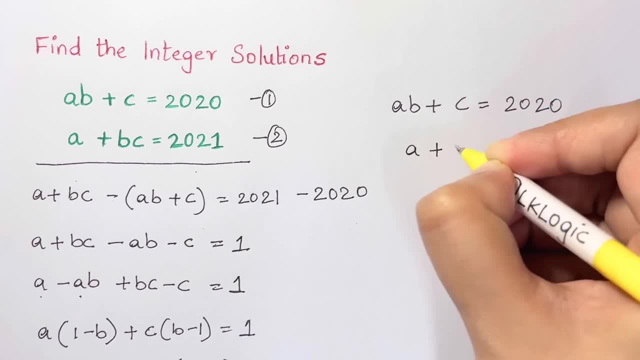 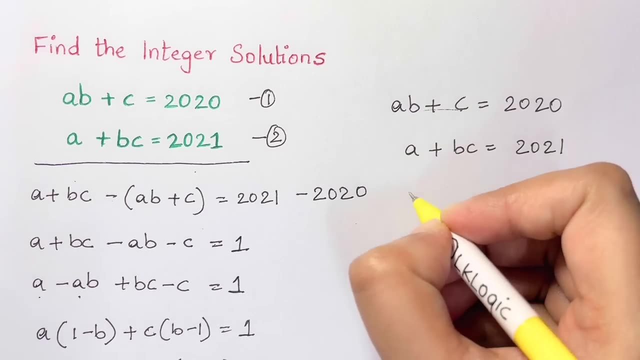 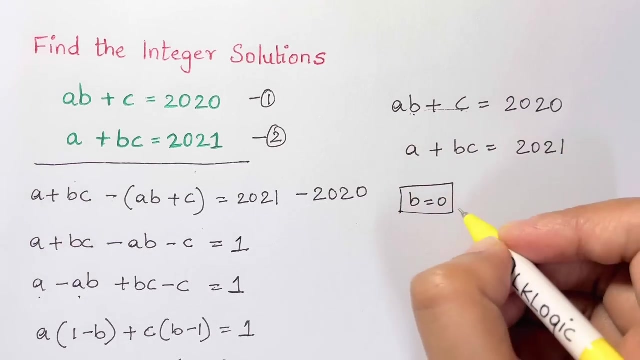 Twenty-twenty And a plus b, c is equal to twenty-twenty-one. If we put b is equal to zero in this, Just put b is equal to zero. So what do we get? b is zero, So c is equal to twenty-twenty. And then what do we get if we put zero in this one? So b is zero. 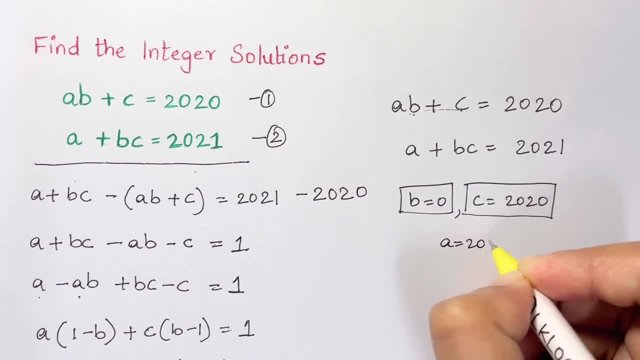 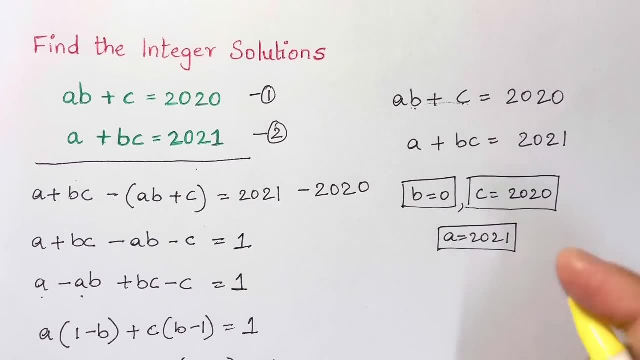 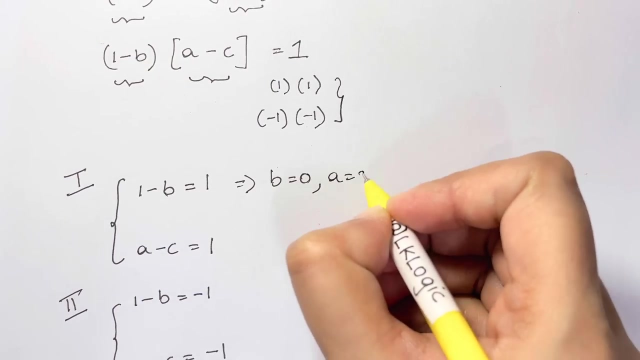 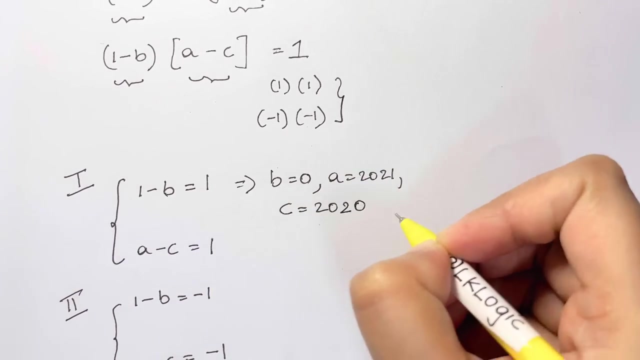 So a is equal to twenty-twenty-one. So we get the three values. Let's write it down: c is twenty-twenty And a is twenty-twenty-one. So let us write it down here: a is twenty-twenty-one And c is twenty-twenty. So this is how we. 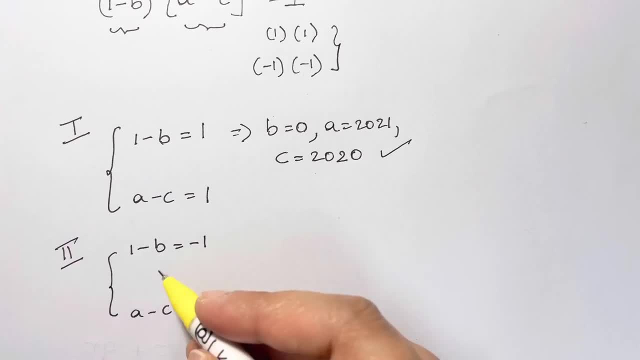 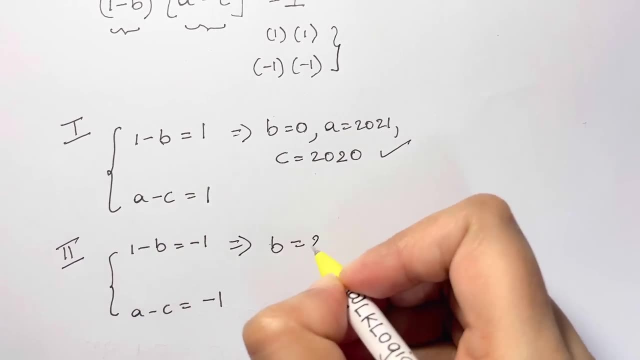 got three values of a, b and c here. Let's find the values of a, b, c here. What do we have? So we have: the value of b is equal to one plus one That is equal to two. So what is? 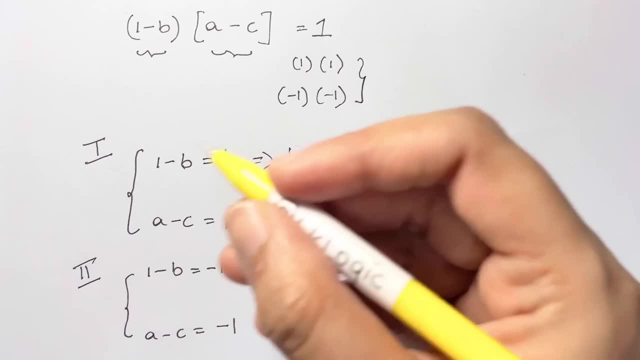 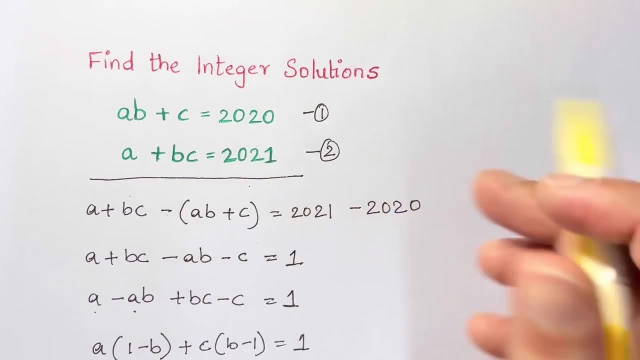 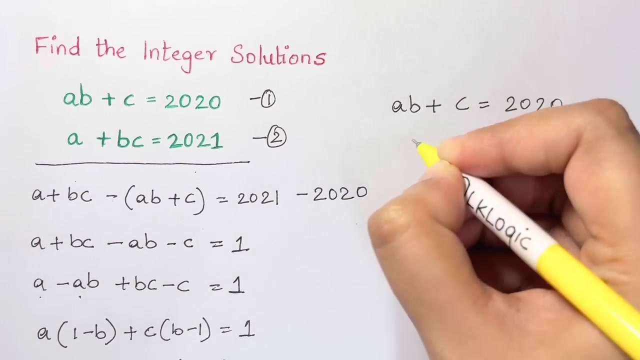 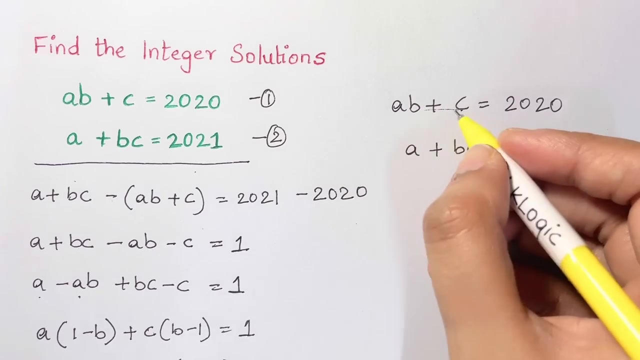 So for that we need to substitute back the value of b in the equations. Substitute back the values of b in this equation. So let's write it down: a, b plus c is equal to 20.. 20 and a plus b, c is equal to 20,, 21.. If we put b is equal to zero in this, just put b is equal to. 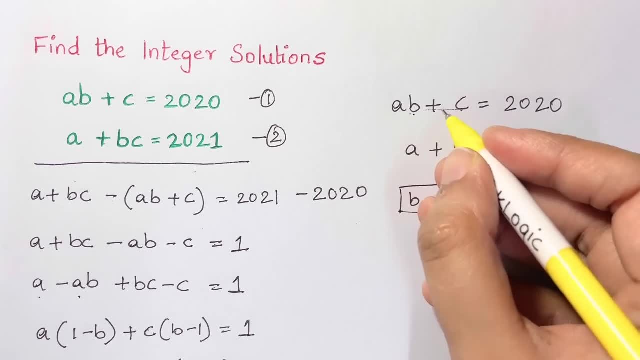 zero. So what do we get? b is zero, So c is equal to 20, 20.. And then what do we get if we put zero in this one? So b is zero, So a is equal to 20, 21.. 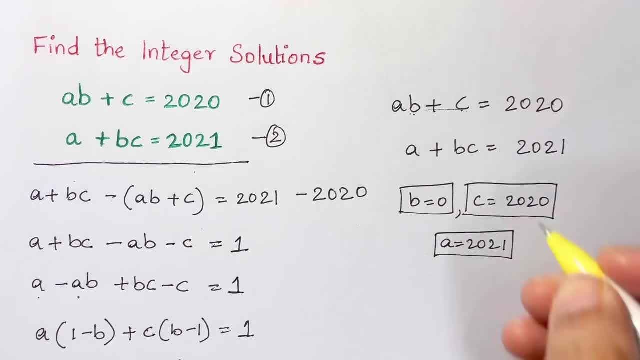 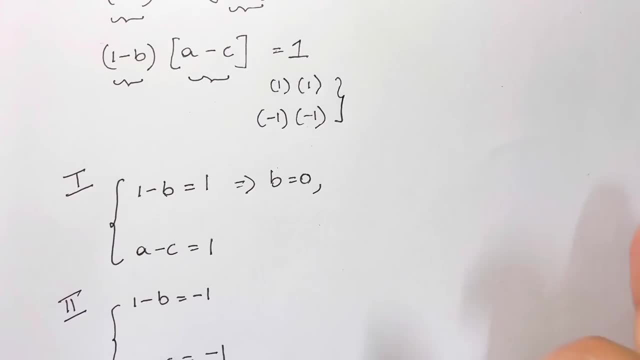 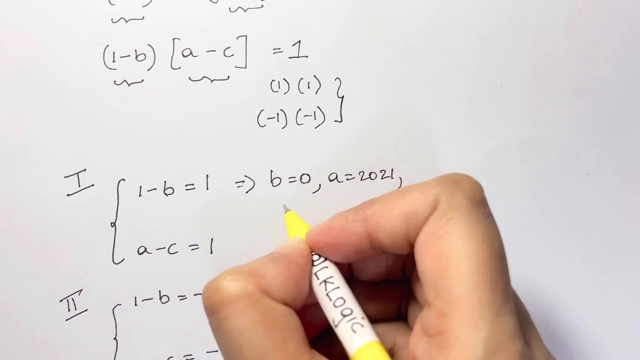 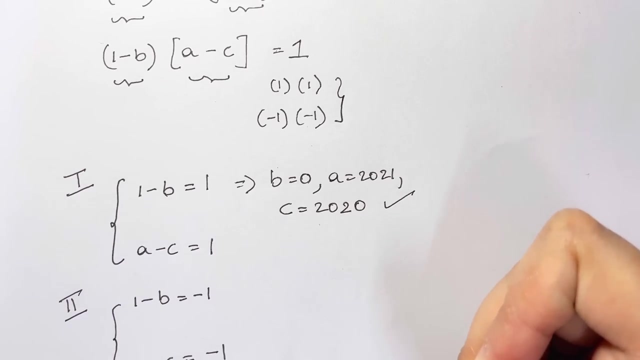 So we get the three values. Let's write it down: c is 20, 20 and b and a is 20, 21.. So let us write it down here: a is 20, 21 and c is 20, 20.. So this is how we got three values of a, b and c here. 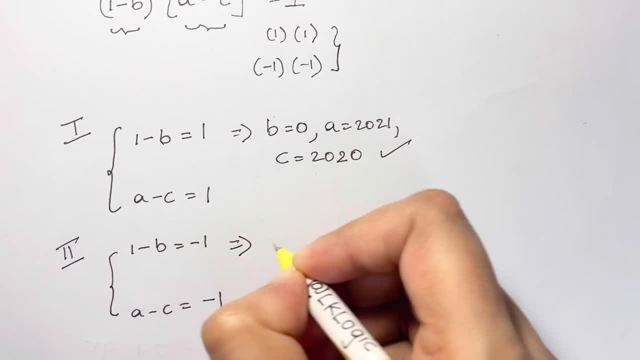 Let's find the values of a, b, c here. What do we have? The value of b is equal to zero. So we get the three values of a, b and c here. What do we have? The value of b is: 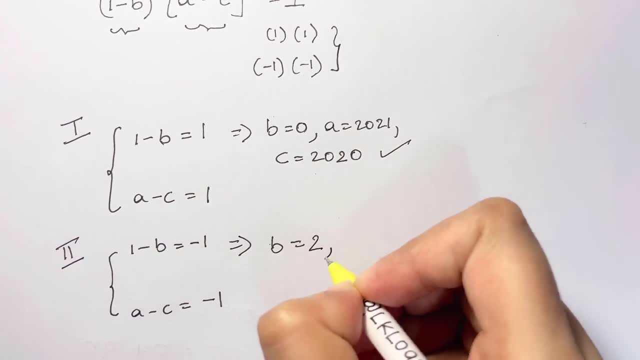 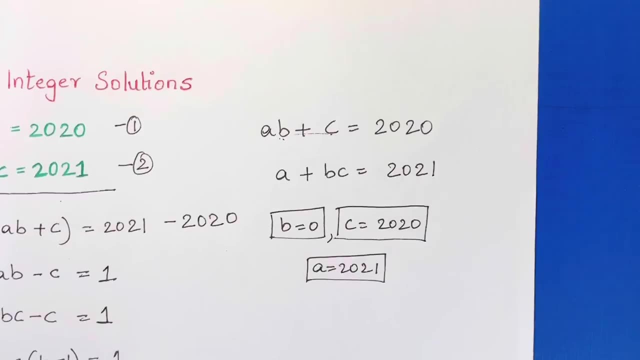 equal to 1 plus 1. That is equal to 2.. So what is the value of a and c here? So let's substitute: b is equal to 2 in the equations. So we have this equation When b is equal to 2, what are the two? 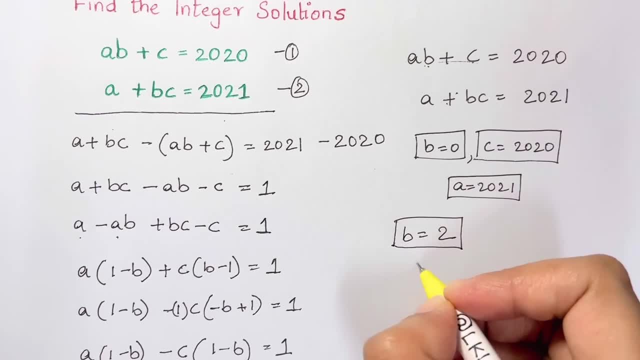 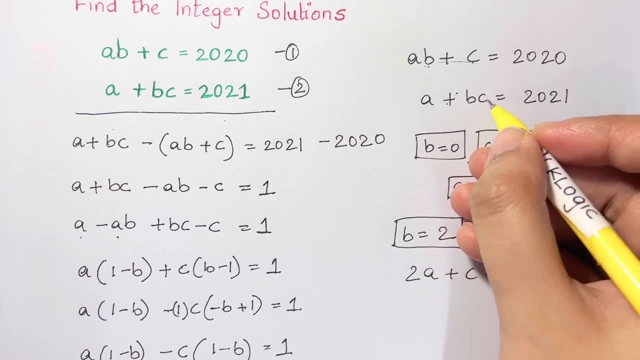 equations: 2a plus c. So I've got: 2a plus c is equal to 20, 20.. And then another one: We have 2c plus a, So a plus 2c, a plus 2c is equal to 20, 20.. And then another one: We have 2c plus a. 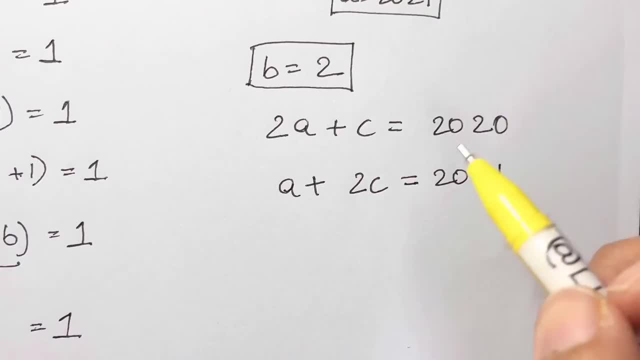 2c is equal to 20, 21.. Now to solve two equations with two variables, either we can use substitution method or we can use elimination method, both. So let's try with elimination method To eliminate a variable. we need to make it same. So we are going to multiply this whole. 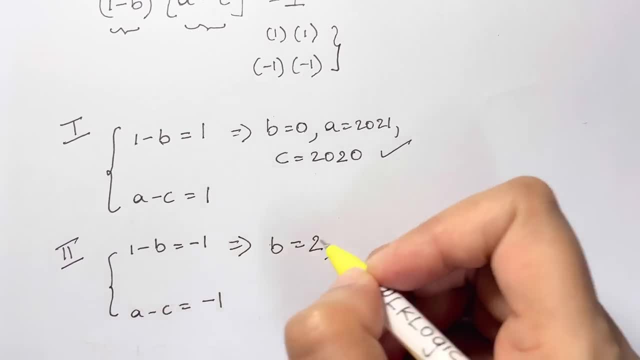 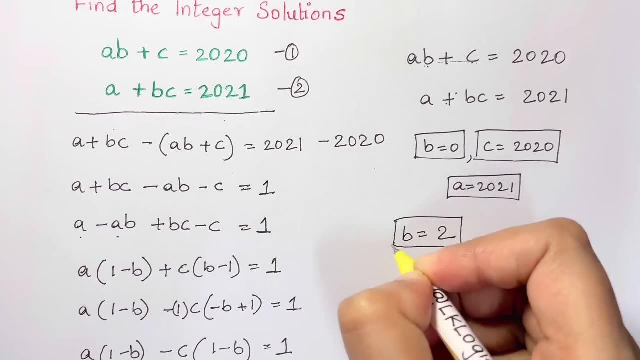 the value of a and c here. So let's substitute: b is equal to two in the equations. So we have this equation When b is equal to two. What are the two equations? Two a plus c. So I've got two a plus c is equal to twenty-twenty. And then another one: We have two c plus a. 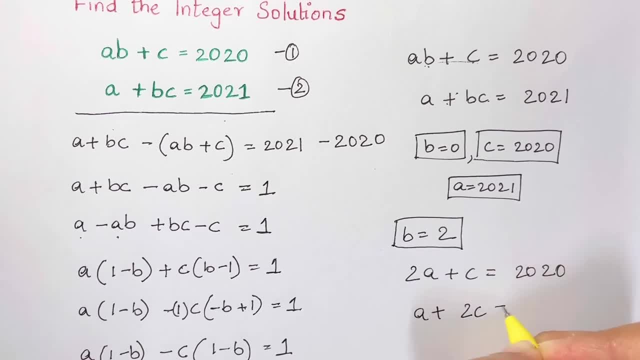 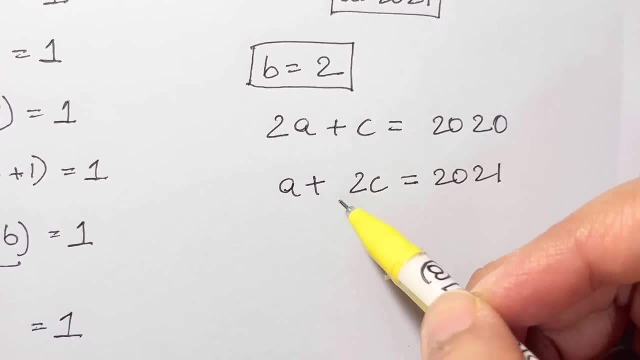 So a plus two, c, a plus c, a plus two, c, a plus c is equal to twenty-twenty-one. Now, to solve two equations with two variables, either we can use substitution method or we can use elimination method, both. So let's try with elimination method To eliminate a variable. we need to make it the same. 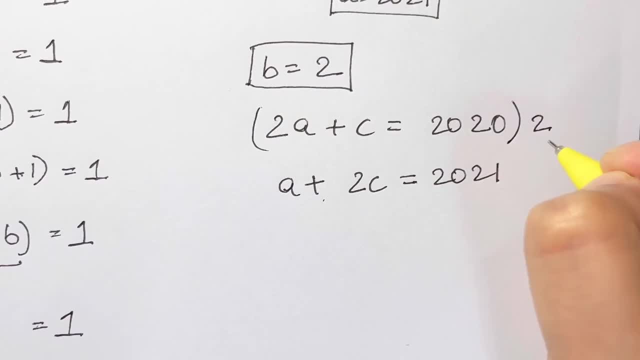 So if we are going to multiply this whole equation by 2.. So what do we get? So we have two times two, That is four a. a is four a plus c to c. plus 2c is equal to 4040. and another equation- i'm going to write that as it is a plus 2c is: 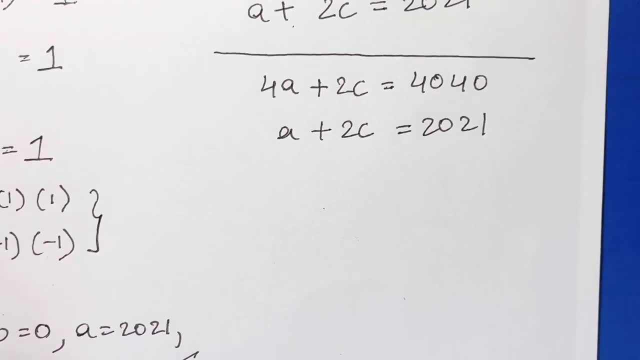 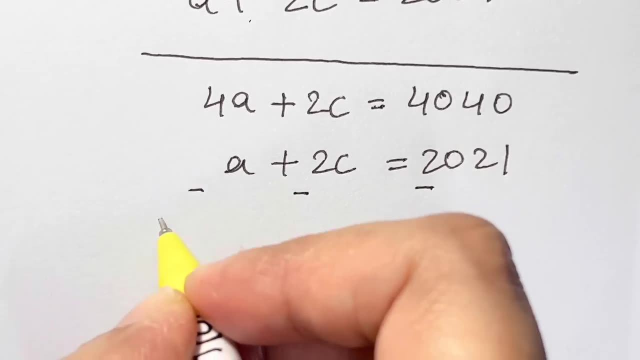 equal to 2021. now we've got two equations to solve. let's solve for that. we can eliminate the variables, just change the signs. 2c gets cancelled. 4a minus a is. 3a is equal to 4040 minus 2021 is. 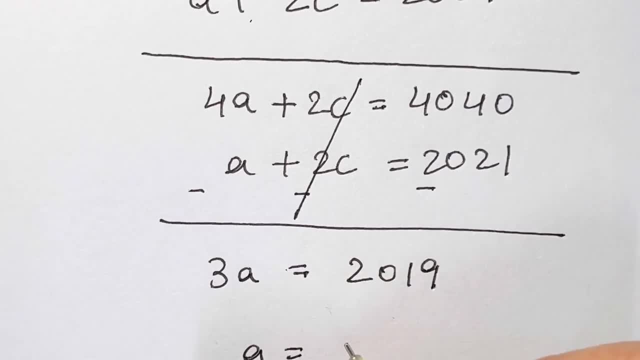 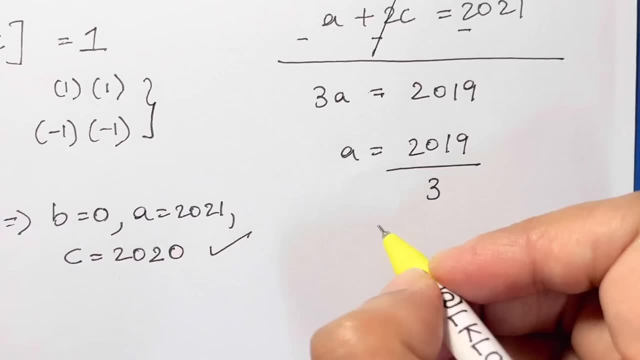 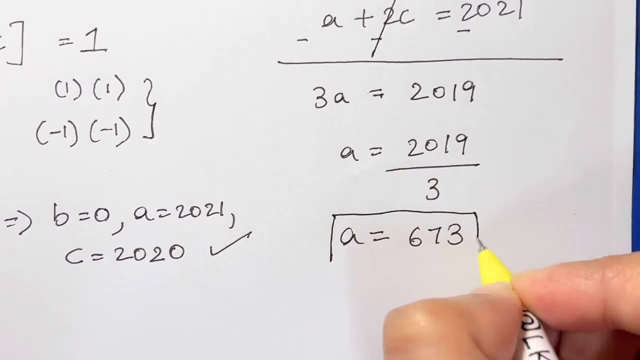 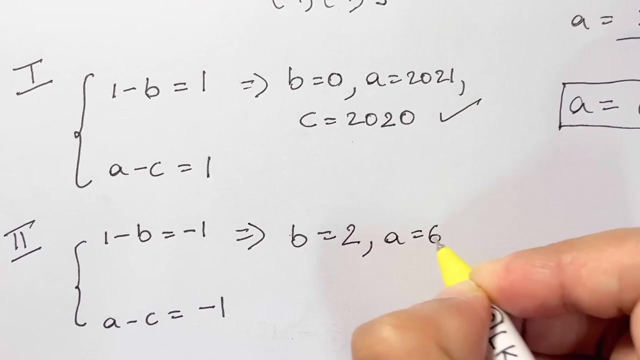 2019. so a is equal to 2019 divided by 3: 29 divided by 3 is equal to 673. now we've got the value of a, so let's put it back. so here we have: a is equal to 673. a minus equals to negative 1. 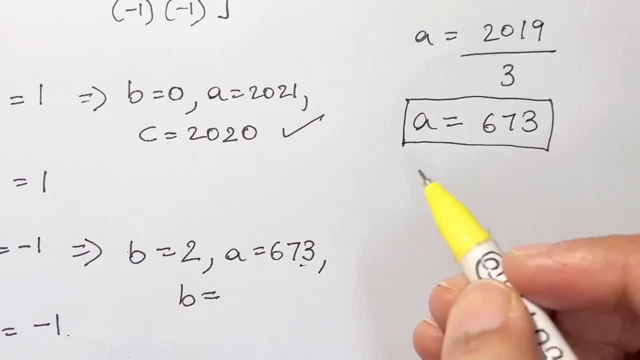 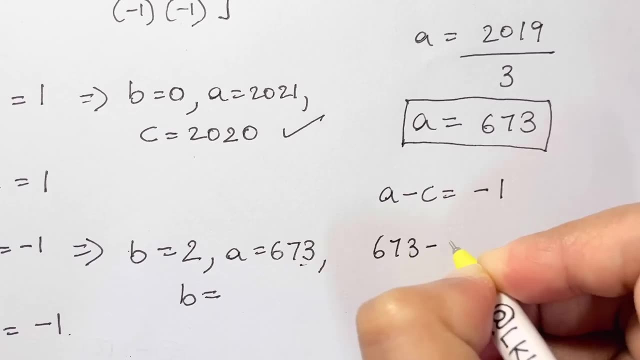 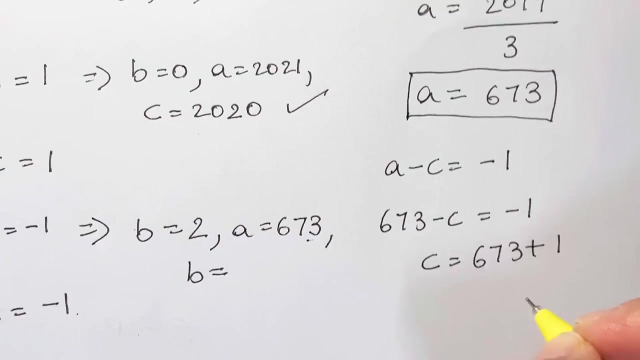 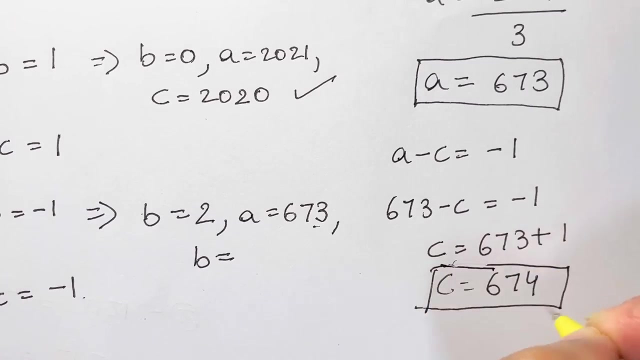 we found the value of a, so let's put it in that a minus c, a minus c is equal to negative 1. a is 673. 673 minus c is equal to negative 1, so c is equal to 673 plus 1, which is equal to 674. so we have got the value of c 674.